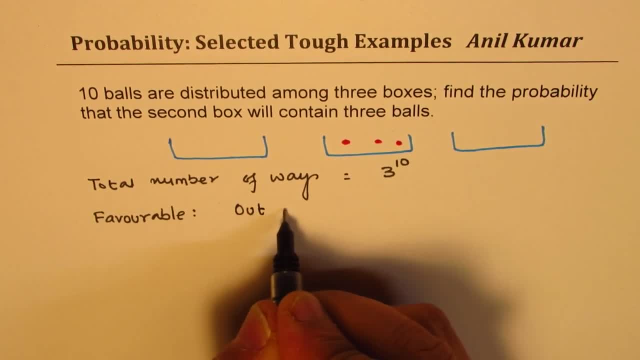 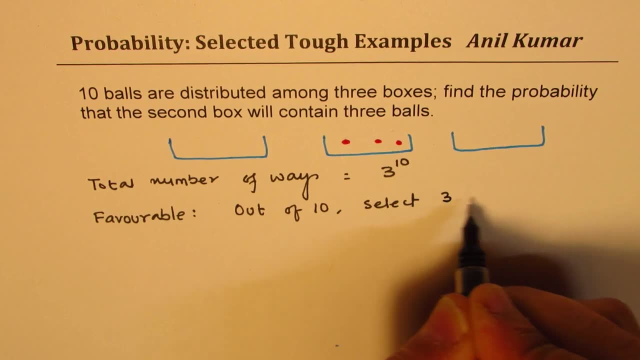 So, out of these 10 balls, so out of these 10, it's Now. you can select three. in how many ways? So that is because they are not distinct right. Any three can come. It is 10C3.. 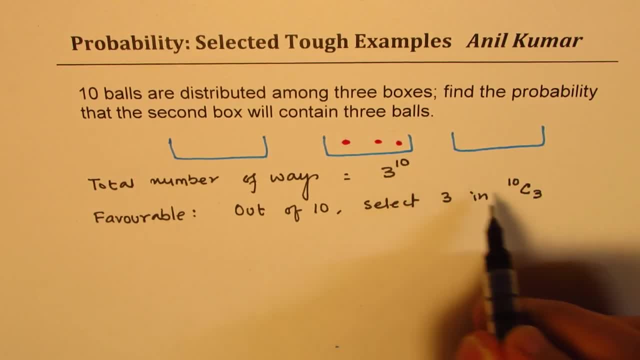 So these are the number of ways. when you select three out of 10 for the second box, right, The rest can go into the other two boxes. So basically, now we have selected three, That means 10 minus 3, which is 7.. 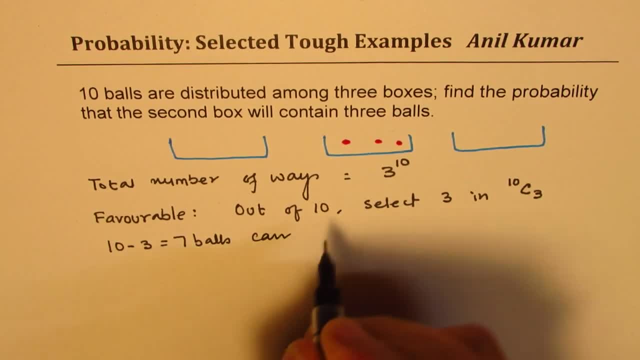 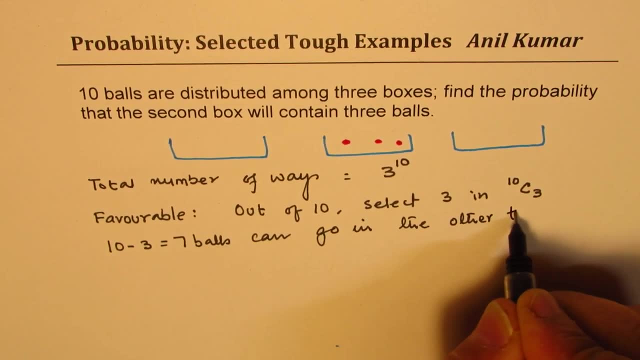 So 7 balls can go in the other two boxes Clear. How many ways are there for those things to happen, For the 7 balls to go into the other two boxes? So when you select these three, 7 will go here. 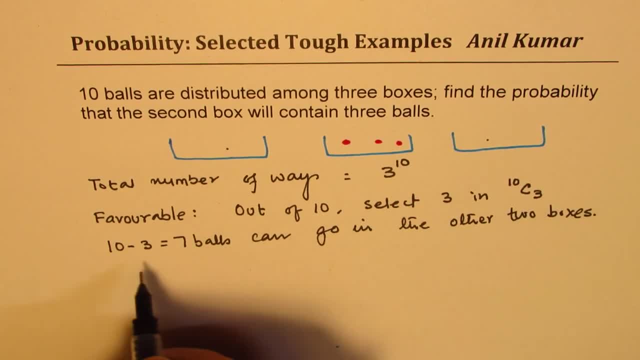 So that is, we have got two boxes and 7 balls. So this is So. this is equal to 2 to the power of 7, right? So the total favorable cases- let's say our event- is A, So the favorable cases for us will be 10C3 times 2 to the power of 7, okay. 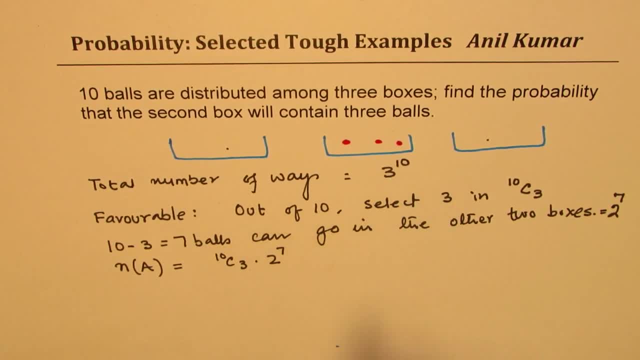 And total number of ways are 3 to the power of 10. And therefore we get the probability as Yes for this particular event, as a ratio of 10C3 times 2 to the power of 7, divided by 3 to the power of 10, correct? 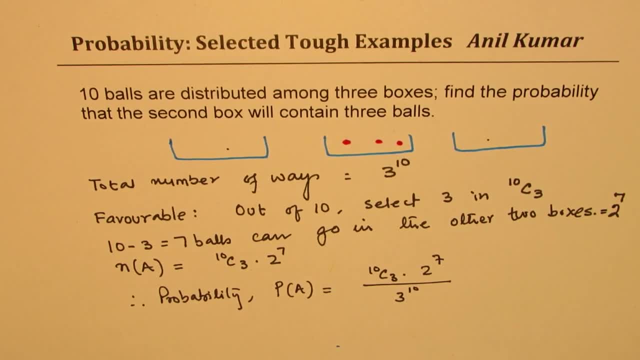 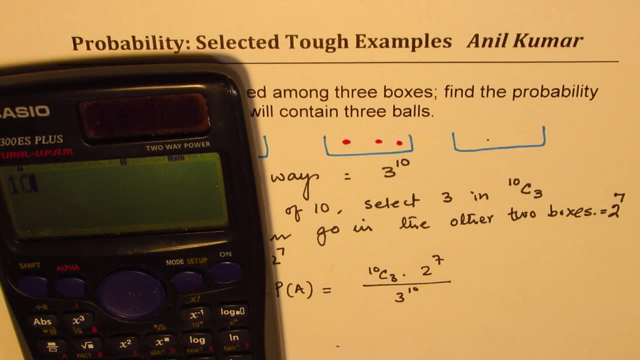 So that is how you could actually find the solution for this question correct. So that's your answer. Well, let's see the number also. So we have 10C3.. So we have 10C3 times 2 to the power of 7.. 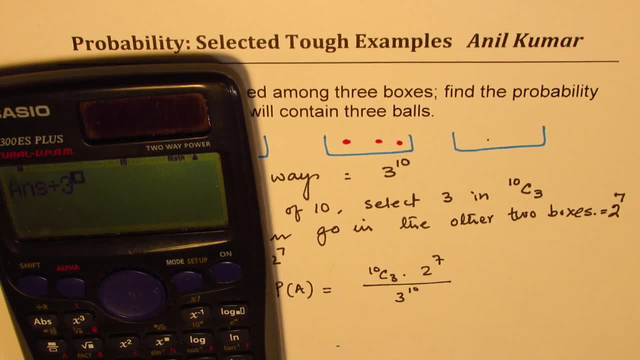 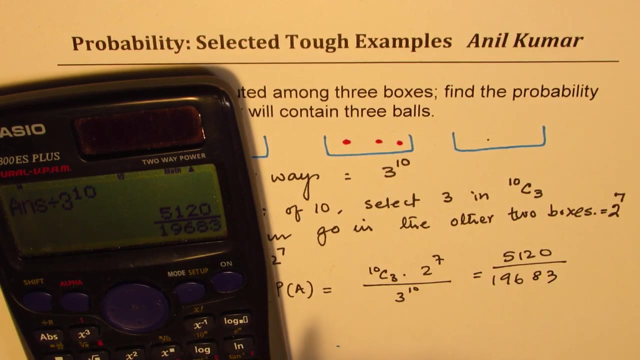 And then we are going to divide this by 3 to the power of 10.. Well, that gives you 5120 over 19683, I think Okay. So the probability is around 26%, which is 0.26..